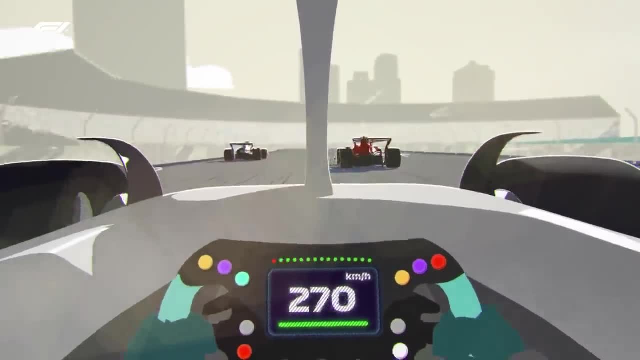 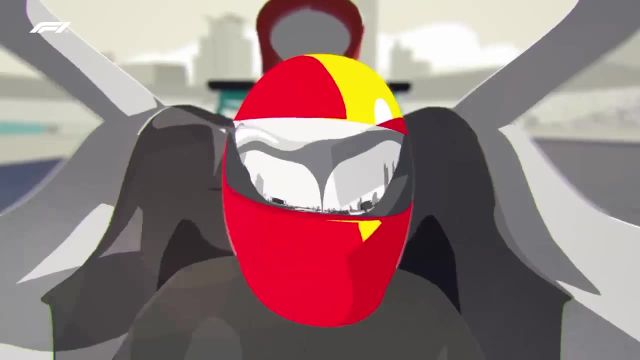 And all at insane speeds. Acceleration: supercars can only dream of top speeds of 370 kilometers per hour and G-forces that only fighter pilots can relate to. F1 is all about pushing the limits of speed, science and nerves. 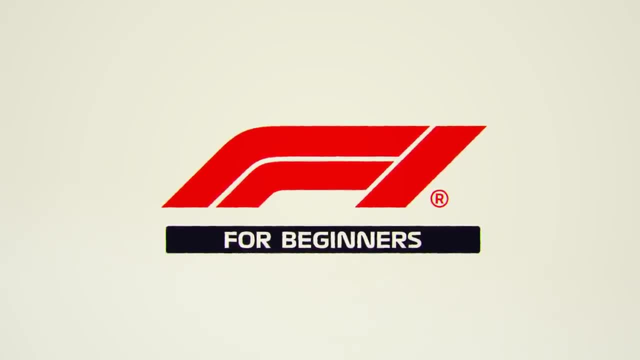 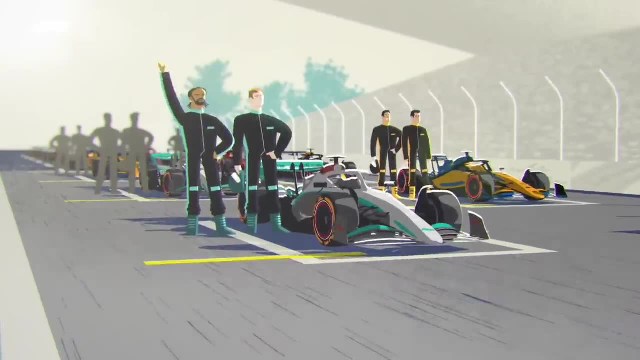 To get you up to speed, here's the complete lowdown on Formula One. It might seem like an individual pursuit, but F1 is a team sport. Currently, 10 teams of two drivers contest each race weekend Referred to as the Grand Prix. 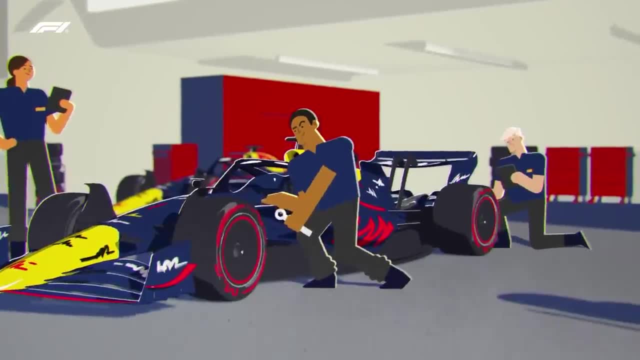 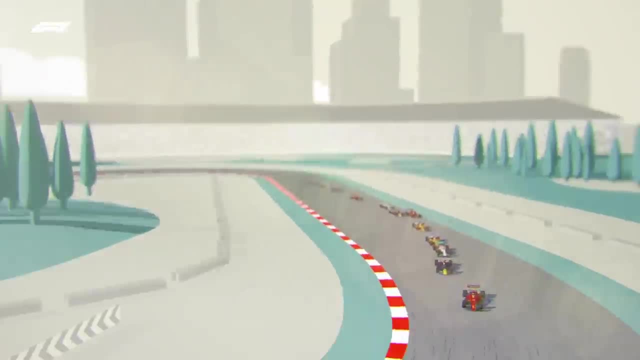 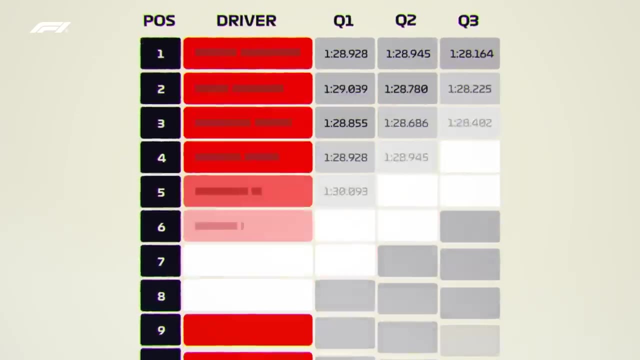 Behind the scenes, each driver is supported by a crew of mechanics, engineers and strategists. to squeeze every bit of performance out of the car. Race weekends start with practice to fine-tune setups before a three-part knockout qualifying session against the clock to determine the order of the driver's lineup on the starting grid. 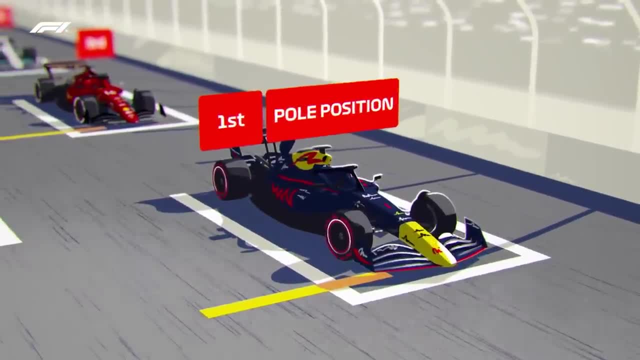 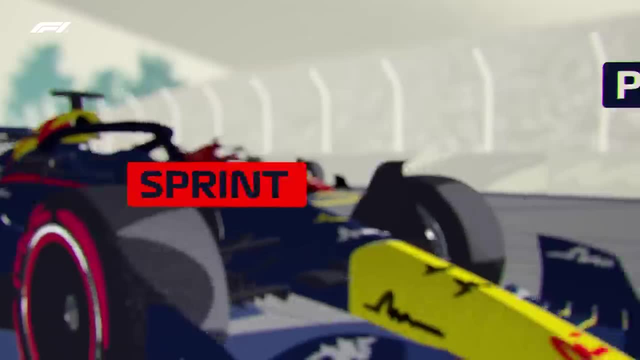 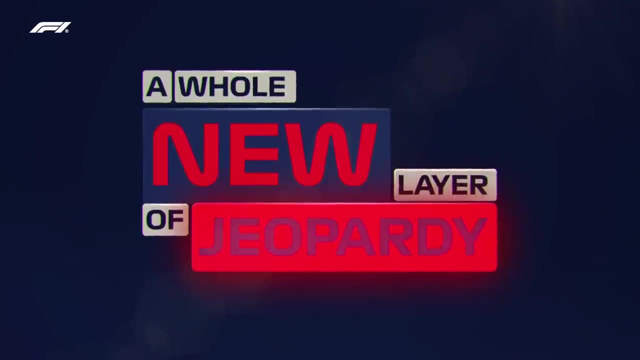 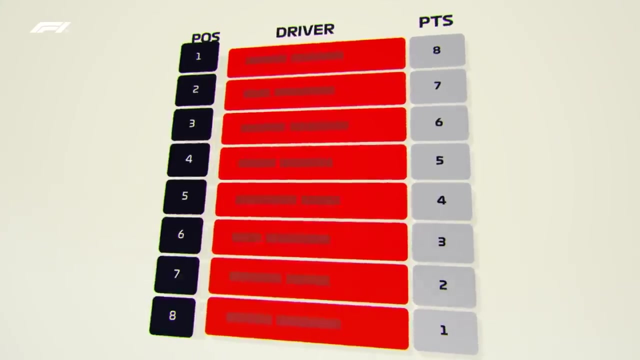 The fastest qualifier starts at the front-end pole position. Certain weekends include F1's sprint event. It gives the fans an extra race between qualifying and the main Grand Prix Run at a third of the full race distance. This adds a whole new layer of jeopardy, with the sprint result not only setting the starting order but also offering points to the top eight finishers. 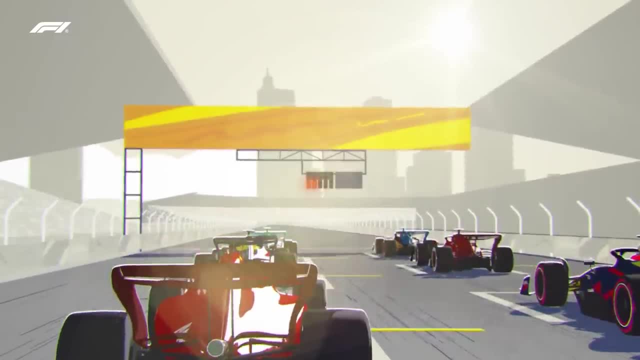 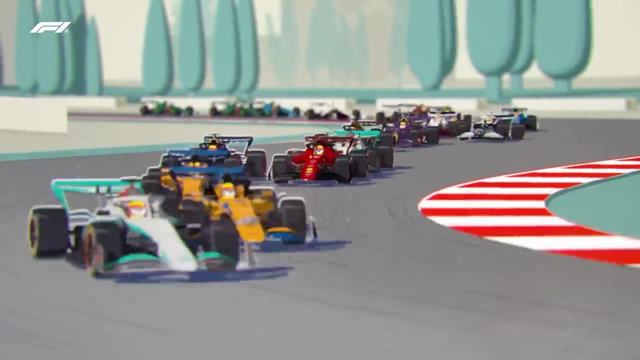 On race day, the five lights come on one by one. before going out to start the race, Drivers muscle their cars around the track, and then the car is ready around the track as fast as possible to reach the checkered flag at the finish line first. 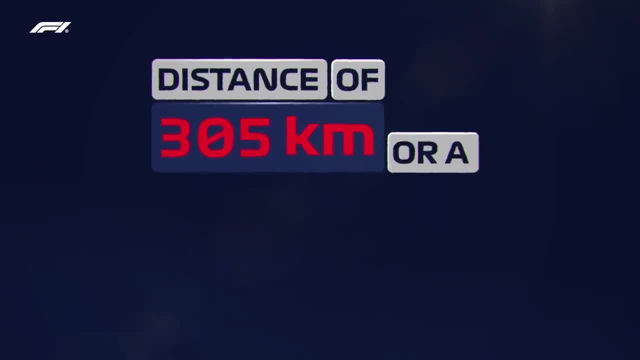 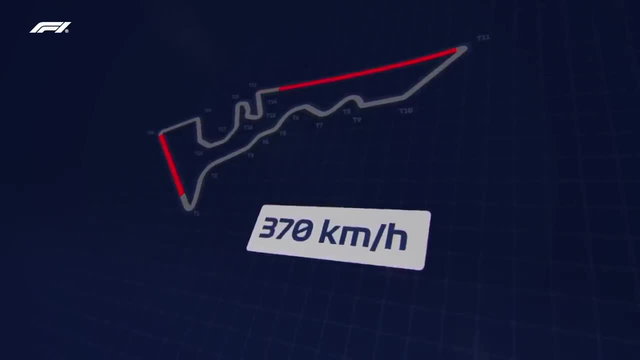 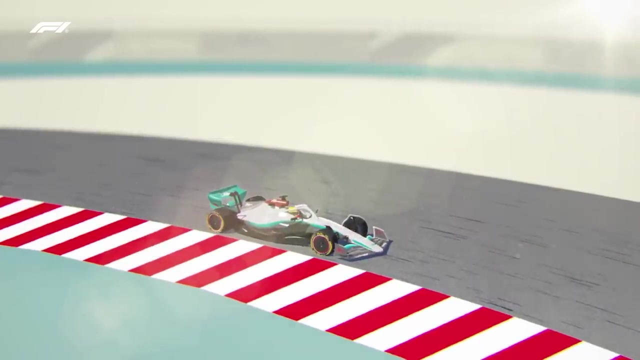 after either a distance of 305 kilometers or a time limit of two hours. At straight line speeds of 370 kilometers per hour, with standing cornering forces of 5G Drivers can corner so fast they experience forces similar to those felt during a space shuttle launch. 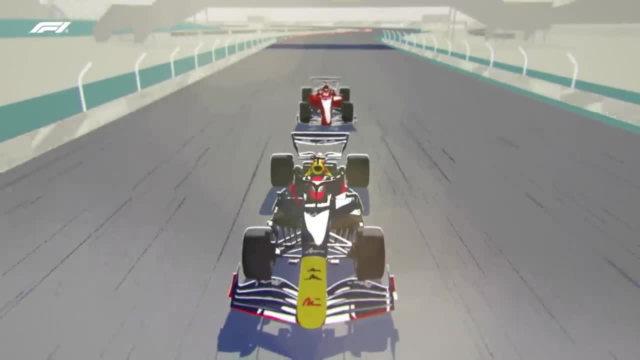 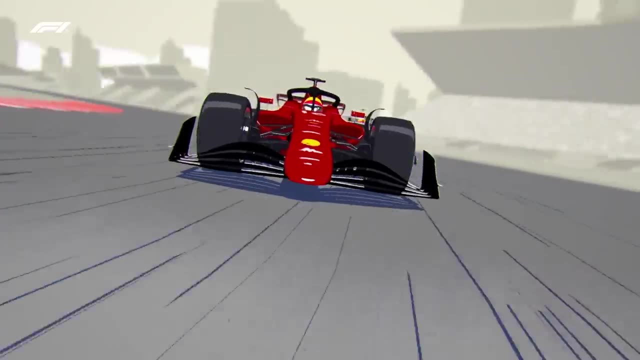 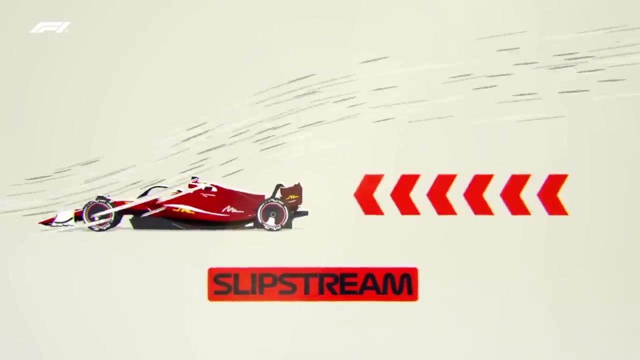 Speed is one thing, but drivers also need to overtake to gain position. F1 races are long and a small braking concentration could present the opportunity to pass or get within the driver's slipstream- an area of disturbed air behind a car that allows a following car to go faster. 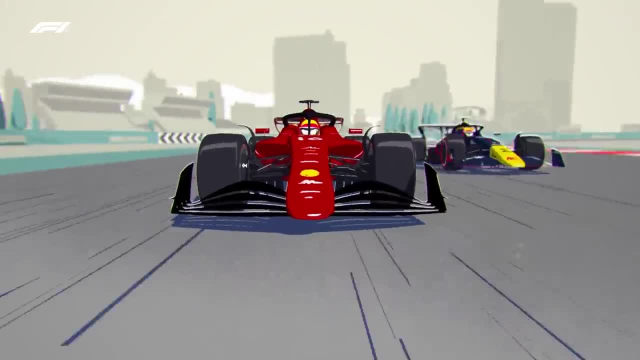 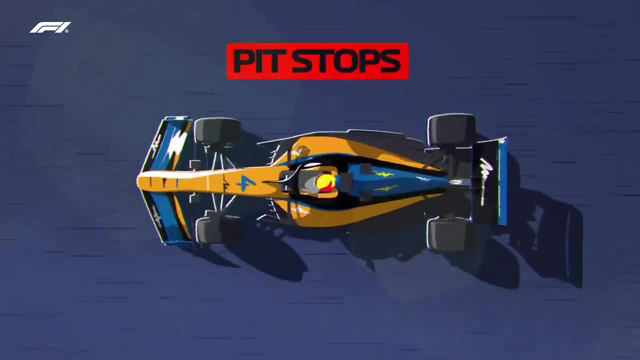 move alongside and pass. This creates incredible battles as drivers jostle to stay ahead for the finish. All drivers have to stop at their garages, known as their pit box, at least once for a change of tires. This task called a pit stop.